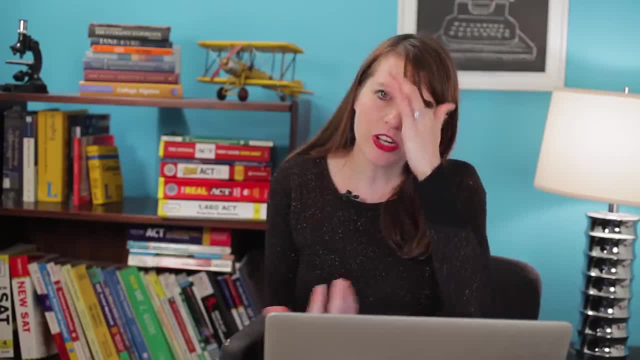 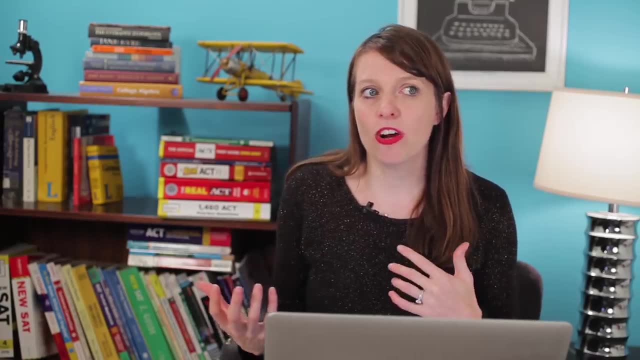 let's get going. So, basically, what I'm going to do today is I'm going to go through some really tough ACT problems. What makes a problem really hard? It might be hard for some of you and it might not be as hard for others of you. Some of it depends, Some of it depends on your. 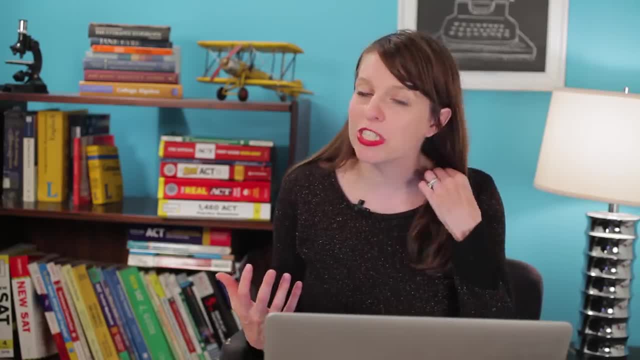 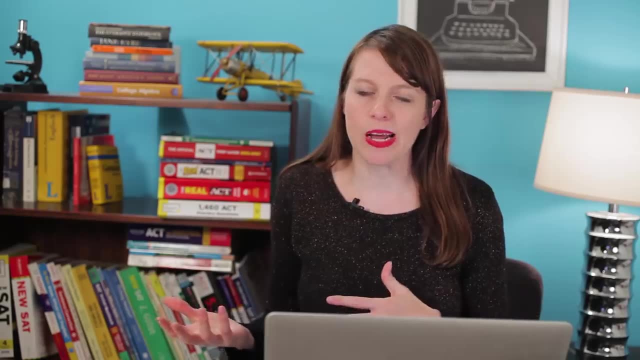 math background is and what kind of math problems you personally are comfortable with versus other problems. So just because these problems might not be super hard for you doesn't mean they're not hard for someone else. I've tried to pick what I find a lot of students tend to struggle with. 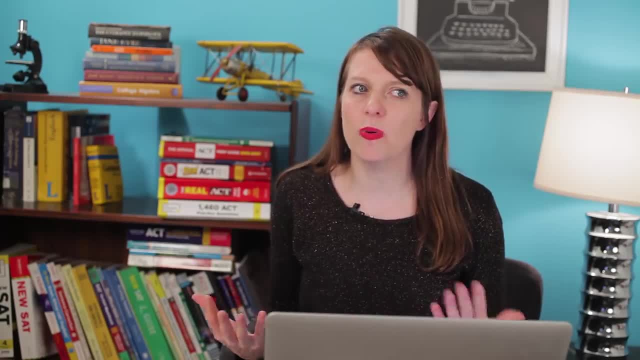 And those tend to be areas that, what I like to say, don't necessarily always fit into traditional math courses. So they might be the kind of problems that you see in probability, statistics, maybe even physics class. They might be the kind of thing that a lot of you just aren't going to see. 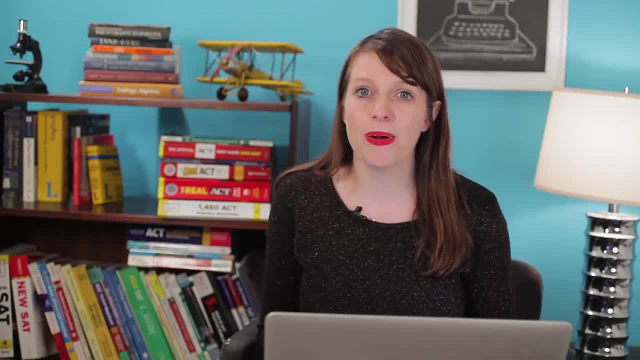 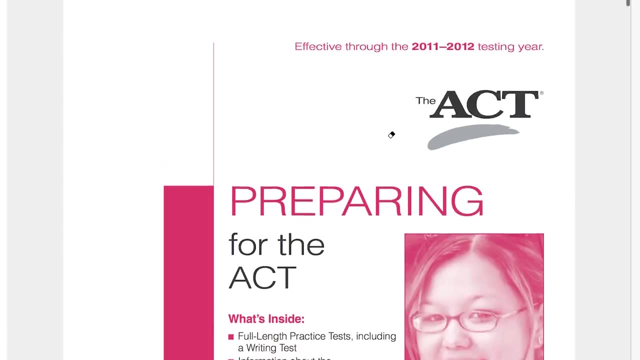 algebra two, or if your teacher gets to the end of the year and runs out of time. These are the kind of problems that your teachers tend to skip over. So that's what we're going to take a look at today. First of all, the source for this. I'm looking in this preparing packet. This is an old 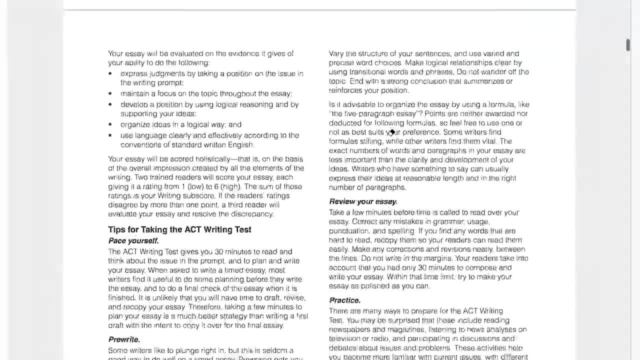 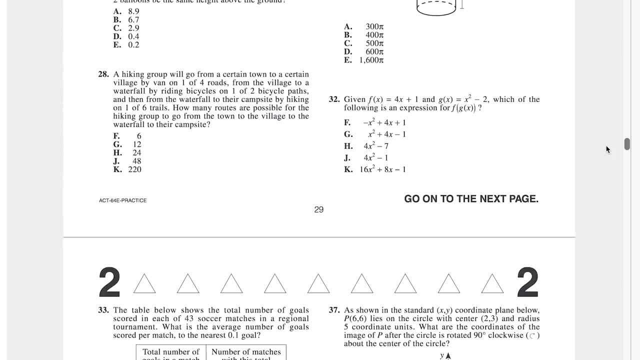 ACT that was offered in 2011 to 2012.. It is form code. If you go off form codes, it's form code 64E. So we're going to go to some of the last problems. So, as most of you probably know, 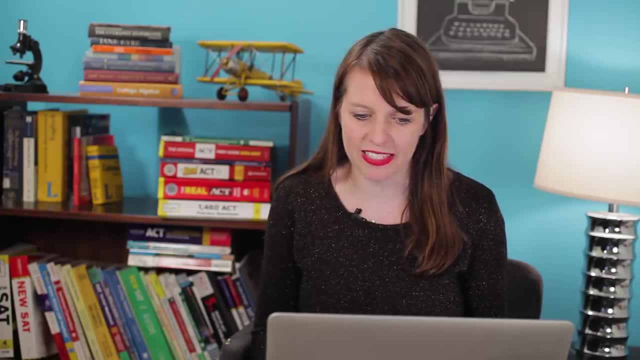 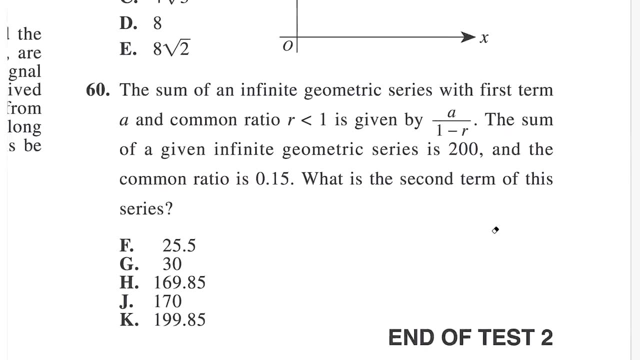 the hardest ACT math problems usually are like the last 10 problems on the test. It's usually where we're going to take care of some of the hardest ones And again I'm going to take a look at some of the hardest ones today, and not only the ones hanging out. So today I'm going to look at some of 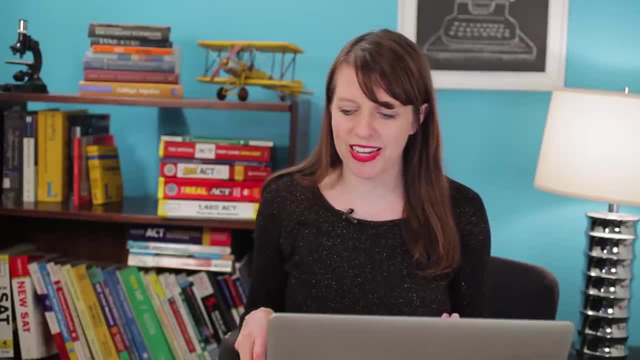 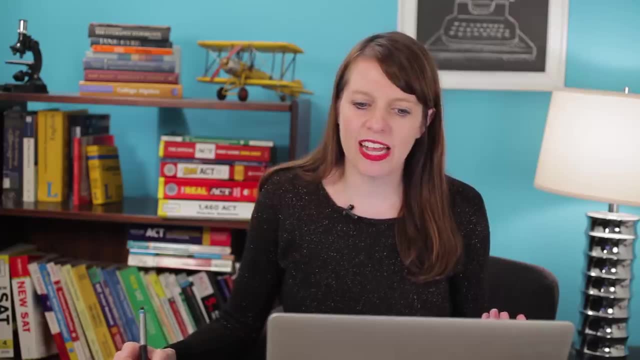 those, And the first one that we're going to do is sequences and series. A lot of people struggle with sequences and series because their math teacher like never taught them how to do a sequence or a series, or they forget what certain kind of series are called, And so that's really confusing. 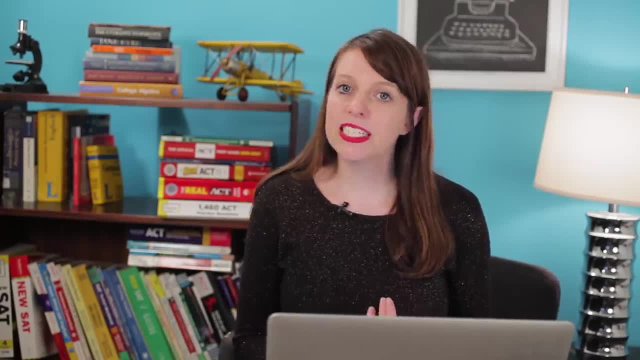 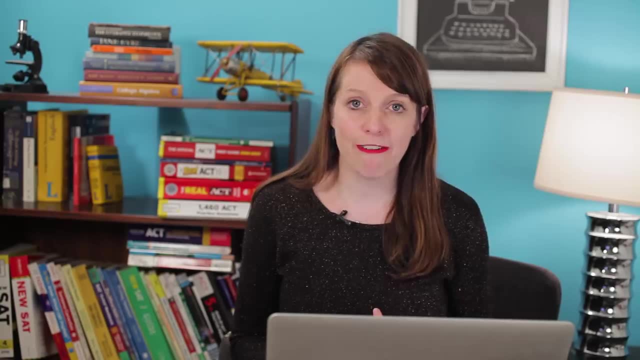 So here, number 60 is a sequence problem. We're going to go over that. If you need more practice on some of these tough math problems, I will say, as part of our best ACT prep course, I will right-click course ever. we do have problem sets that cover almost every section of the ACT math section. 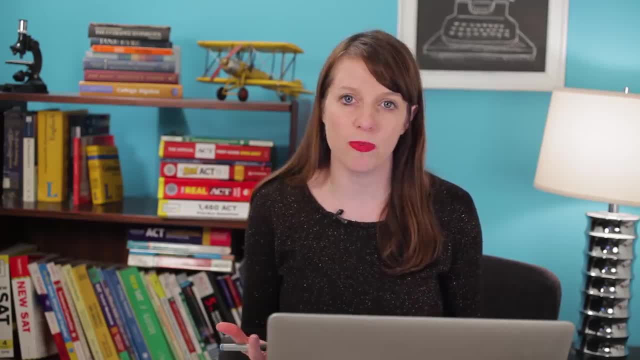 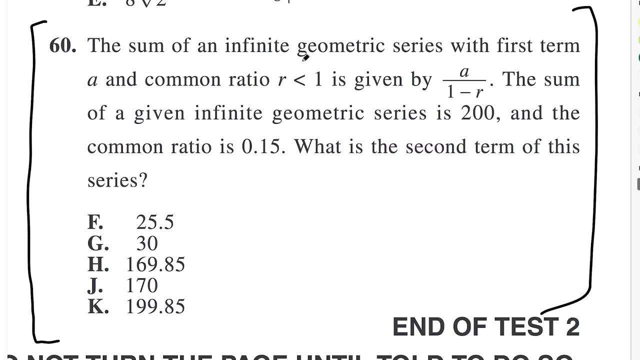 including sequences and series. We have a whole problem set full of these that's available to our subscribers. So if you do want more practice on these, I recommend that you go check that out. So let's go ahead and take a look at number 60.. The sum of an infinite geometric series with the 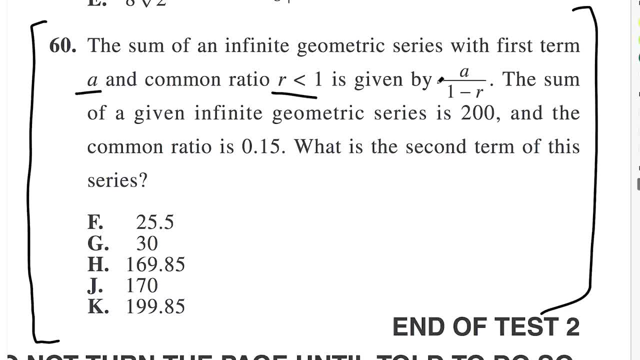 first term a and common ratio r is less than 1 is given by a over 1 minus r. The sum of a given infinite geometric series is 200 and the common ratio is 0.15.. What is the second term of the series? So to get this question right you have to do two things. One, this is kind of what I call. 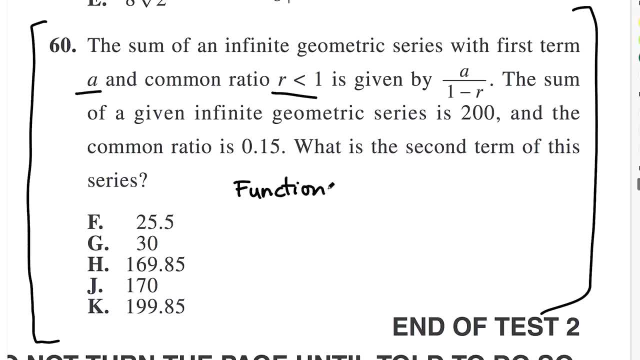 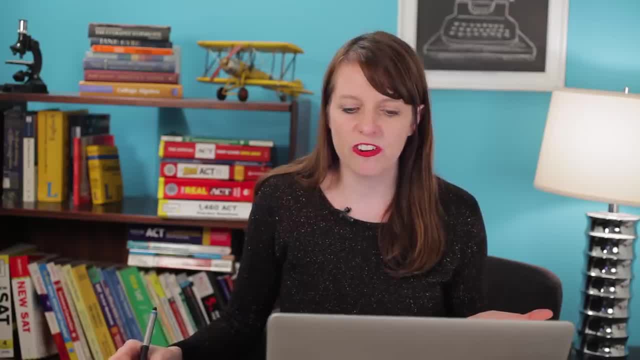 a function as a model problem. This is sort of like a mixed problem, meaning it's a little bit of one type of problem and a little bit of another type of problem. So not only is it a sequence and series problem- right, It's about an infinite geometric series- It's also what I call a function. 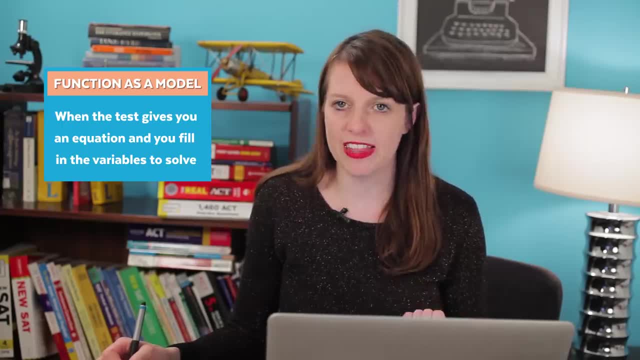 as a model problem, meaning that they give you an equation and they give you a function as a model problem. So if you do that, you're going to get a little bit and you have to fill in that equation with what you know. So let's first start with this equation. 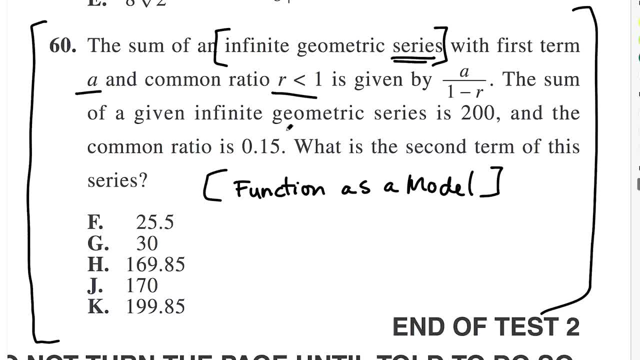 or expression that we're given and we're going to fill in what we know. So what we know is: the sum is 200, right? So I'm going to say 200 equals a over 1 minus r, Cool. And then I know that the 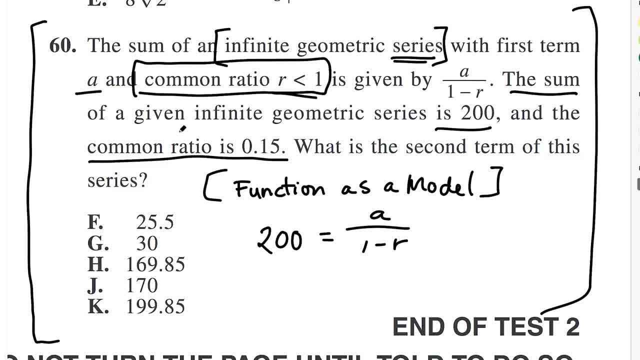 common ratio is 0.15, and this is common ratio. r is less than 1.. So 0.15 is r. Okay, And so that goes right here. So I can say: that equals a over 1 minus 0.15.. Got it, So this just basically becomes 0.85.. So I get 200 equals a over 0.85.. 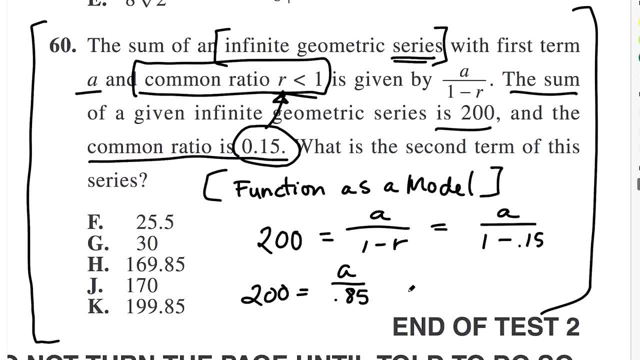 Okay, And now all I do is multiply both sides by 0.85 and that gives me 85 plus 85, which is 170 equals a, And I would recommend you can just get out your calculator and do that math, if it's. 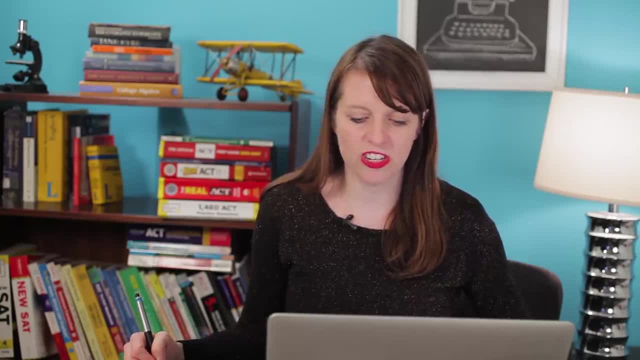 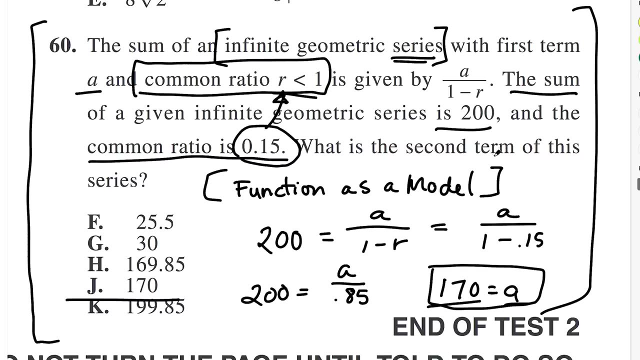 any strain to the brain or just so you make sure you don't make any mistakes. That's usually a good idea. So I get 170 equals a, but guess what? That is not the question- One of the big mistakes that people make, or why ACT problems can be super hard, or why a hard ACP problem is hard. 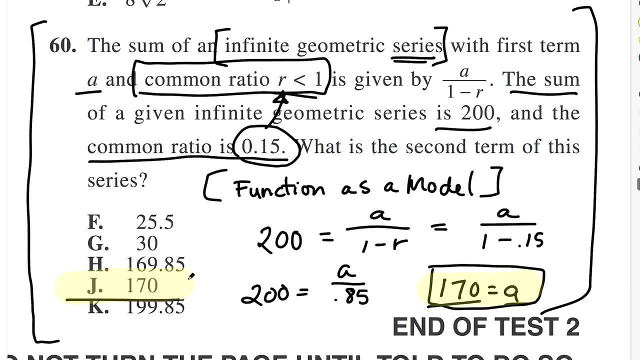 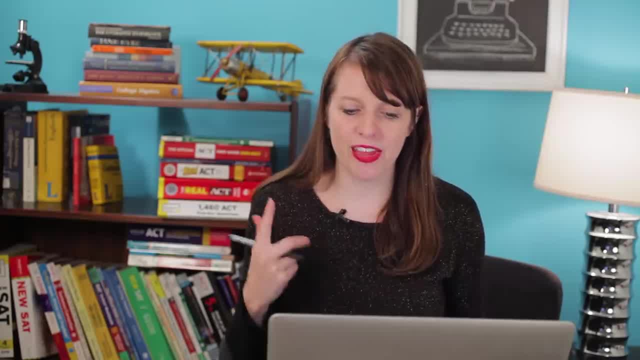 is that the interstitial math that you're doing? you get to this end point and you're super excited and you're like, yeah, I got the answer. You're not done yet. It's probably a two-step problem. So that's my first tip: When you have these tough problems, make sure you read the question. 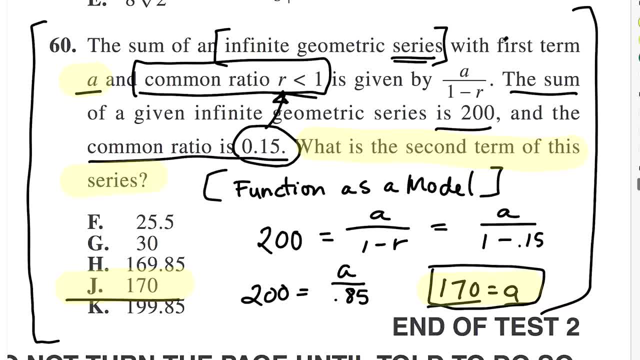 What we actually mean is the second term of the sequence. Guess what a is. A is the first term. Then, in order to get the second term, you actually have to know the definition of a geometric series. If you don't know that or forgot it, you are screwed. So I'm going to 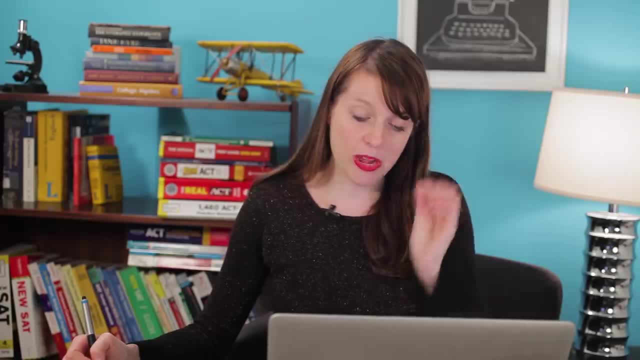 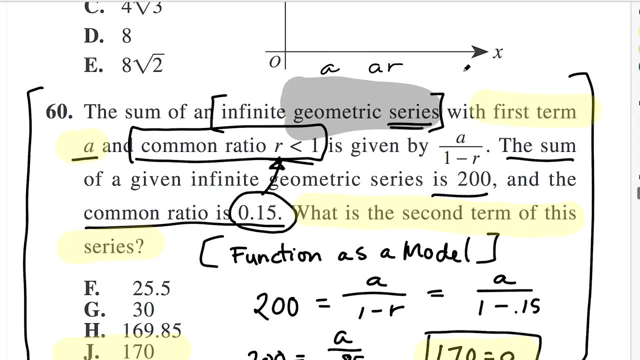 review with you what a geometric series is. A geometric series is a series in which we have like a first term, like a, and then we multiply by r each time to get the next terms. So, for example, my first term would be a, my second term would be a r right, My third term. 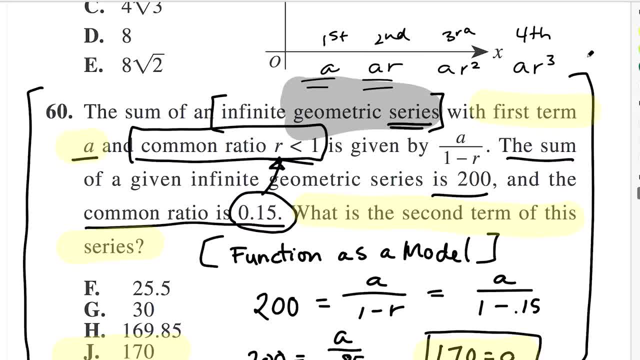 would be a r. My fourth term would be a r- cubed, et cetera, et cetera. Okay, So that's like the situation, That's how it works, And what's going on here is r is 0.15.. So my first term is 170, right? 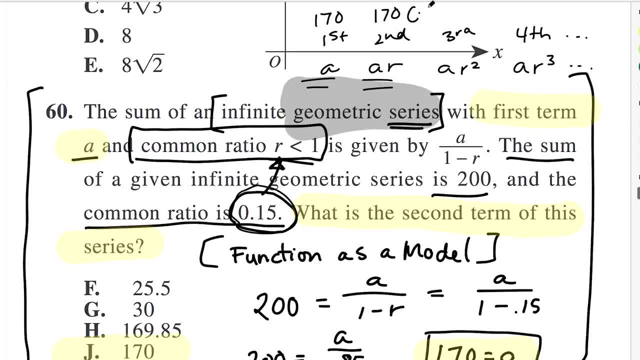 My second term is going to be 170 times my common ratio times 0.15.. Okay, And so what you do is you do 170 times 0.15 and you get 25.5.. Okay, So this is 25.5.. 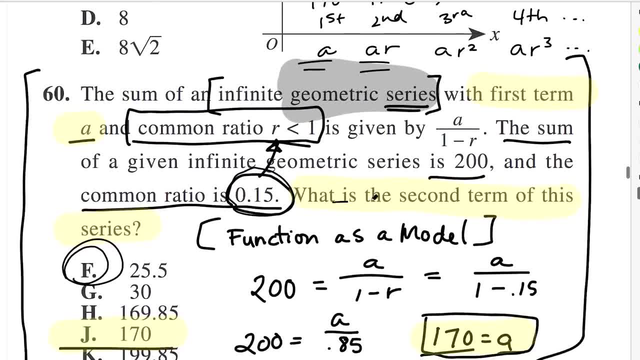 And that is actually the answer, because it's the second term in the series. Okay, So two things you have to know here. First, you have to do this function as a model stuff, which just means you have to read this equation, understand what it means and then plug in all the stuff, But the 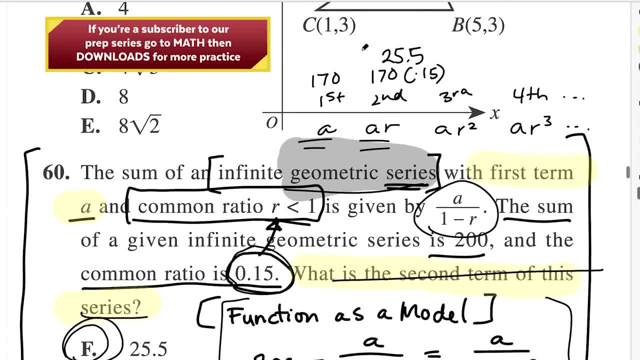 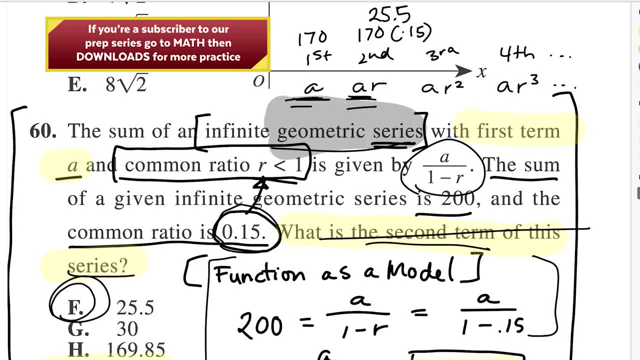 second thing you have to know is what the heck is a geometric series, and how do I then calculate the second term if I know the first term and the second term is just the first term times that common ratio? There's another kind of series you need to know about as well. That's the 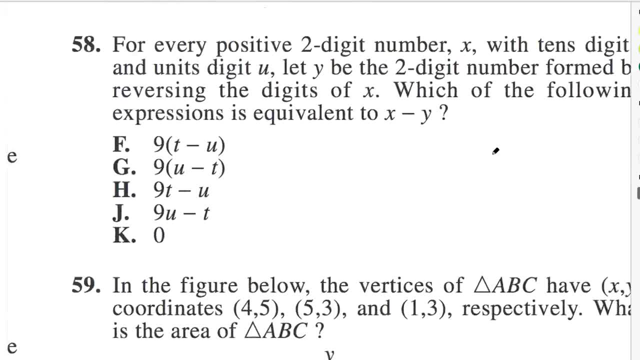 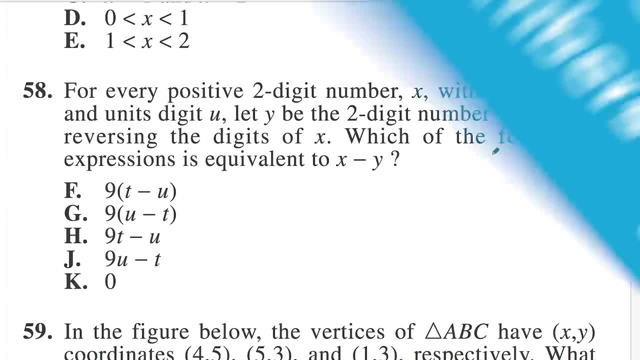 arithmetic sequence Next. So this is another question that's kind of tough that my students struggle with And I would call this what I call. this is a properties of numbers question, And the reason I call it properties of numbers question is it has to do with, like integers, 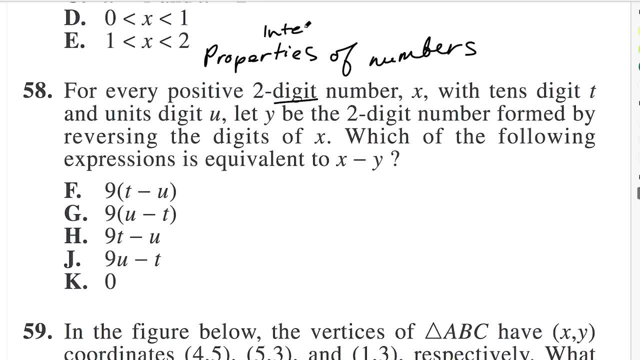 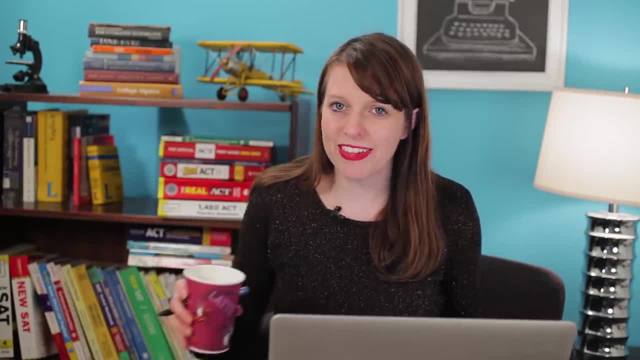 primes and digits right Whenever you see a word like integer, a word like prime or a word like digit, these kinds of questions can really stump students, because they're the kind of thing that, like most math teachers don't necessarily teach There's, they don't. 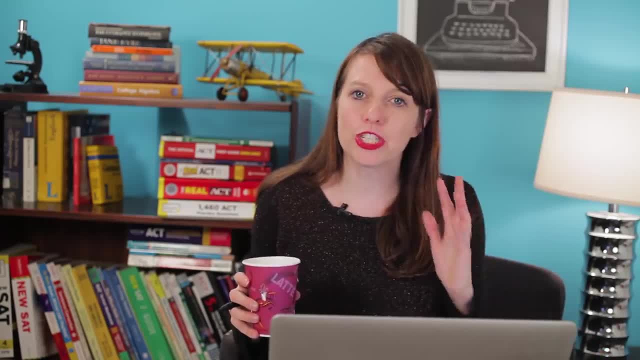 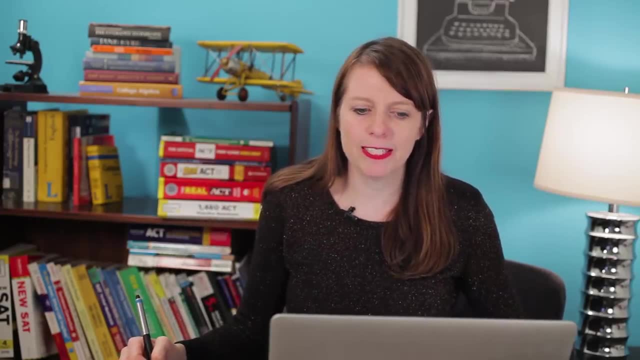 quite fit into algebra. I mean, there are algebraic questions, but they're not straight algebra, right, They're not quite geometry. So therefore they're this kind of question that a lot of you struggle with, simply because you don't see them in math class that often. So let's talk. 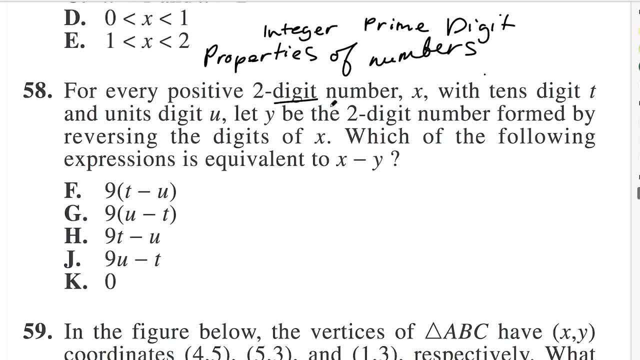 about how do we approach this. one For every positive two digit number X, with tens digit T and units digit U, let Y be the two digit number formed by reversing the digits of X. So let's just wrap our brains around that What that means is we have a two digit number, X, right? 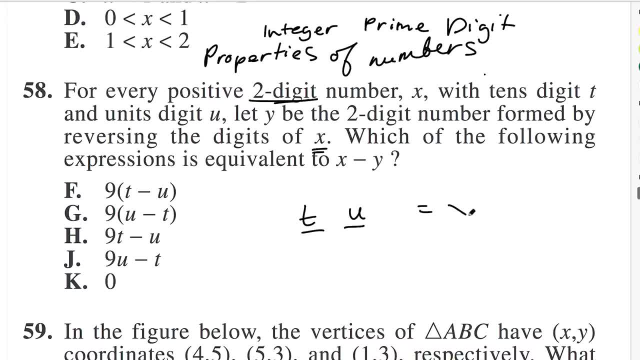 And X looks like this: It's T then U, right. Then we have a digit, a Y, and it's the two digit number formed by reversing the digits. So that's U then T, right, This is tens and ones. 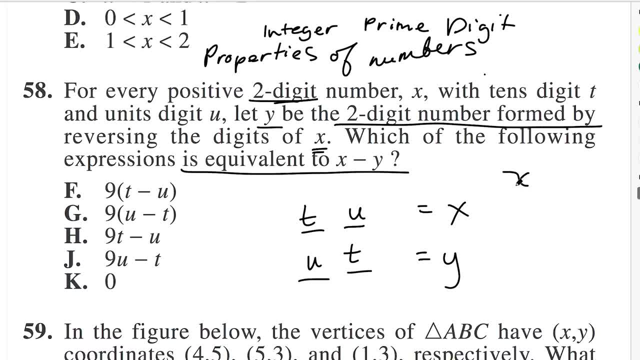 Which of the following expressions is equivalent to X minus Y. So here's what I want. I want X minus Y. Well, this looks and sounds really confusing, but actually it's a lot easier than you know, because what we can do is we can represent these with algebra. Okay, Let's talk. 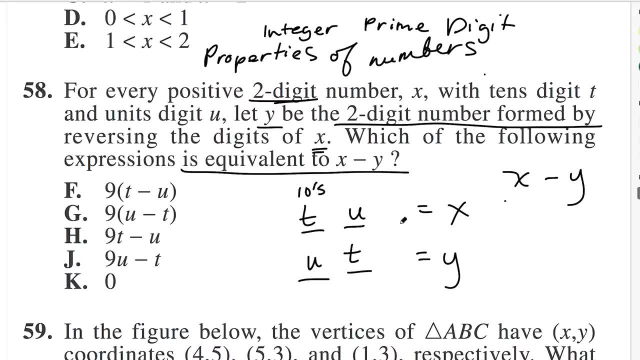 about how we do this, because this is the tens place. I could actually find the value of this. This was 35, right? How do I represent 35?? Well, that's three times 10 plus five, right? You see how I'm using the idea of the tens place to use this digit to then turn that into the value that 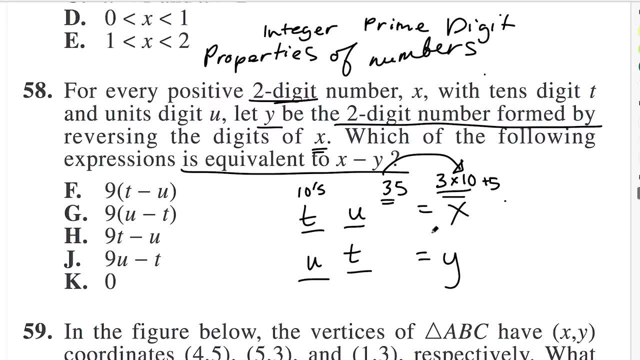 that digit represents, which is three times 10, right? So this, essentially, if I want to say what that is, that is 10 T plus U. Do you see how? this is the value of X? right, It's 10 times whatever. 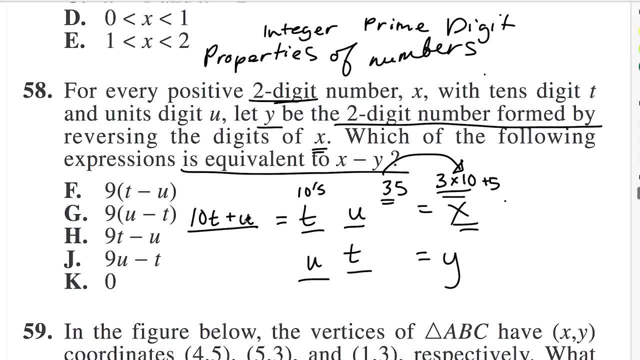 this is: If it were a three, it would be three times 10.. And then we're going to add the units digit onto the end, right? And we do the same thing down here. So this is 10 U plus T, right? 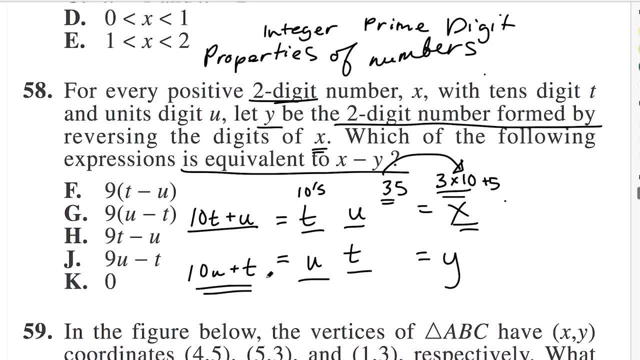 You see how I can represent this algebraically, And this is just a fun trick that we can pull with these digit problems. You can just remember: whenever you have digits or place value, you can multiply by 10 or by a hundred or by a thousand or the other way, If you have points. 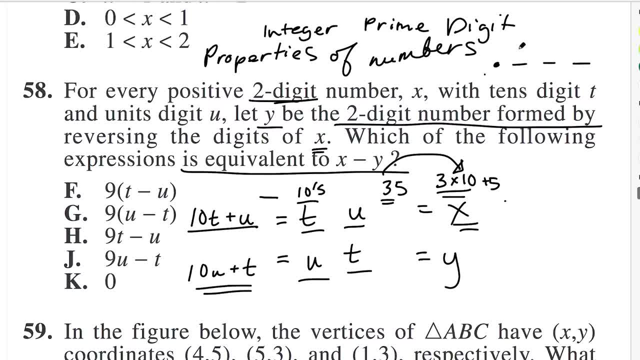 something, something, something you can multiply, right? You can divide, divide this by 10, right Divided by 10, here divided by a hundred, If you have these two digits, right, Et cetera, This could work either way, Even if we're after a decimal. 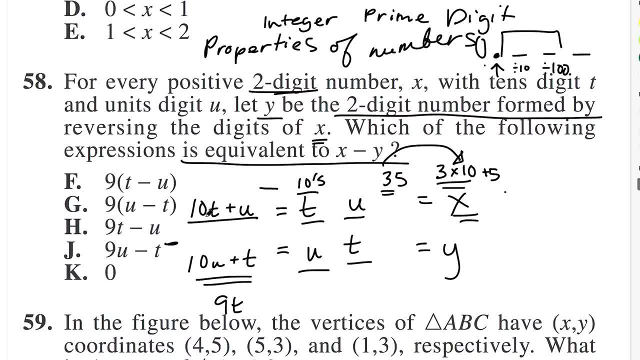 point. we can use the same technique and make this concept into algebra, And then we just subtract our algebra that we came up with and I get nine T right, Cause this minus this, and then U minus 10, U is negative nine U. So nine T minus nine U. 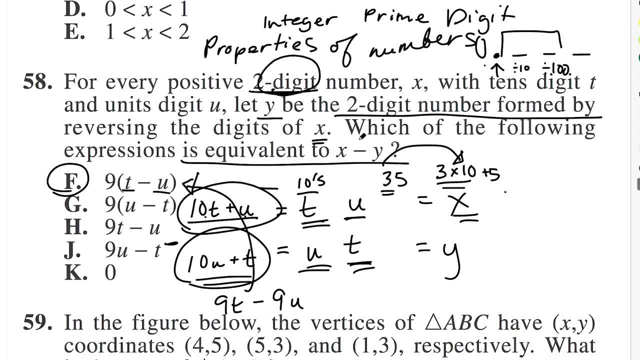 and so there it is, T minus U. It's just factored up here. But you can see, it's really easy if we can kind of get to this point where we recognize how do we shift from the idea of digits to the idea of numbers. It's not impossible, but there you have it. That's all I'm going to go through. 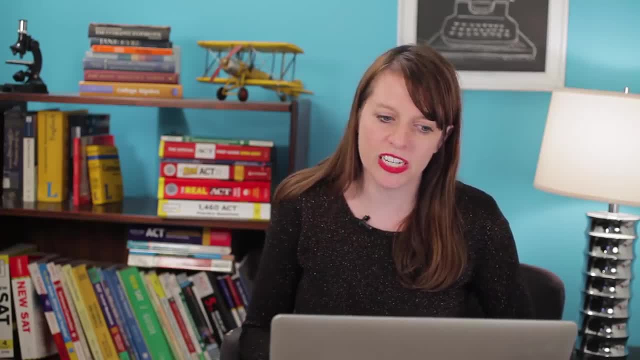 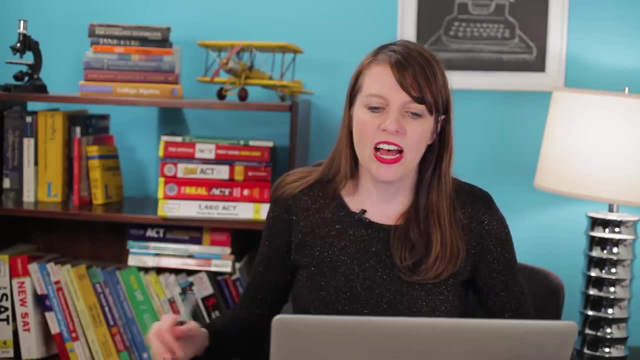 for right now. But what I am going to talk about is, if you are struggling with math on the ACT, what are some other kinds of problems that you should be aware of or work on? So I'm just going to talk about some of the areas that most of my students struggle with. And, again, if you're a 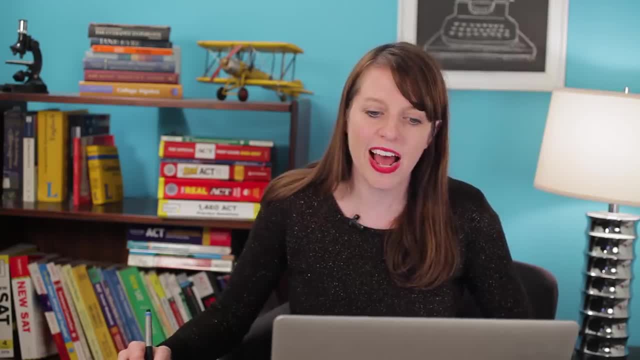 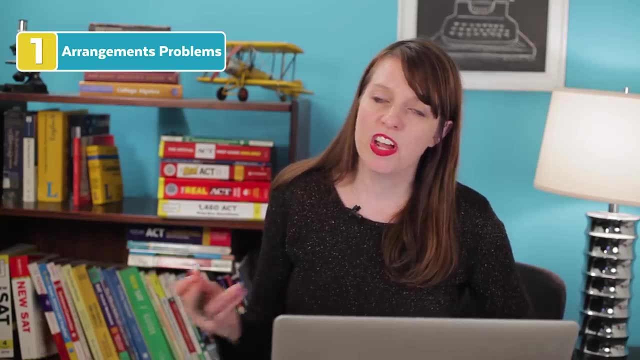 subscriber to our course. we have packets on all these that you can review, And if you're not, you can just like get on the internet and make sure that you know how to do these kinds of problems. One arrangements problems are a big kind of problem that I see people have issues. 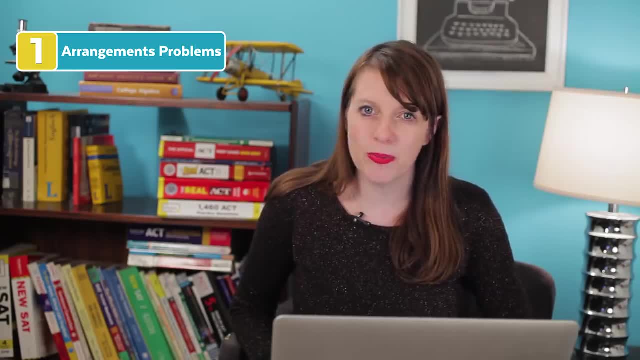 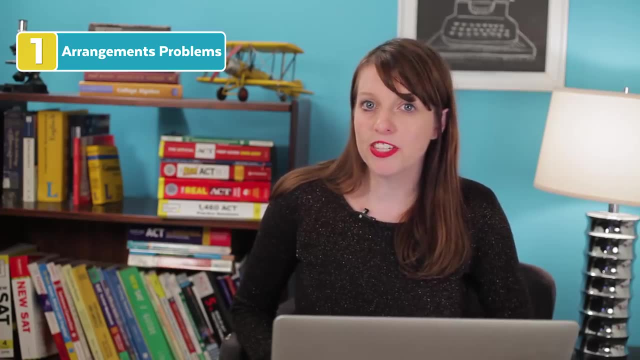 with. Those are like permutations and combinations. Sometimes those fall a little bit under probability and statistics, but permutations, combinations and arrangements, that's a type of problem that you need to know that many of my students struggle with. Another kind of problem: 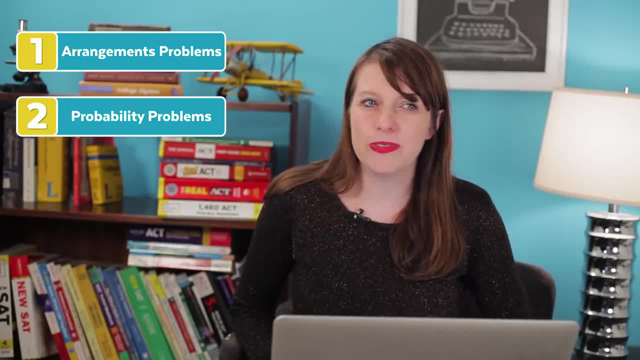 students struggle with is probability problems, mostly because, again, like you see that in stats, but a lot of you haven't taken statistics, So you might not be super awesome at probability, And that's something to watch out for. Those have also been increased in quantity on the test As of. 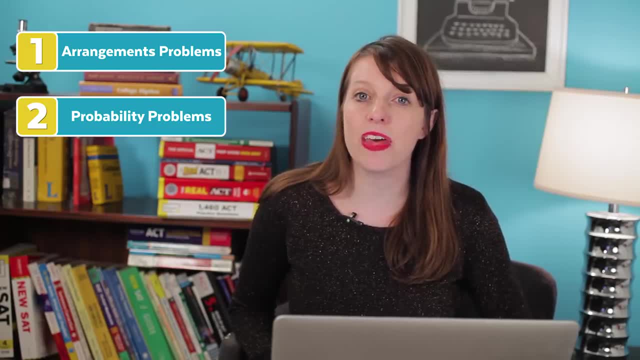 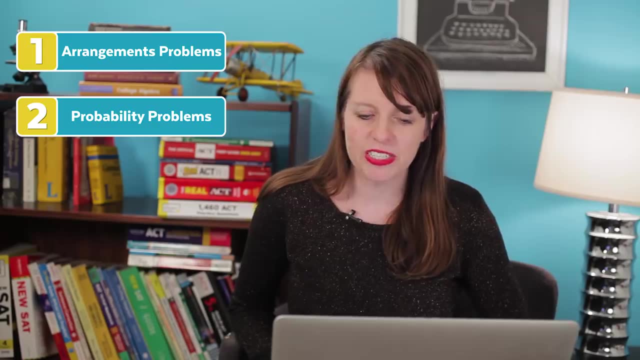 2014,. there are many more items on the exam now that deal with probability and statistics than there used to be, And so I found that that's a bit of an Achilles heel for many of my students, And also if they're working with older prep materials. 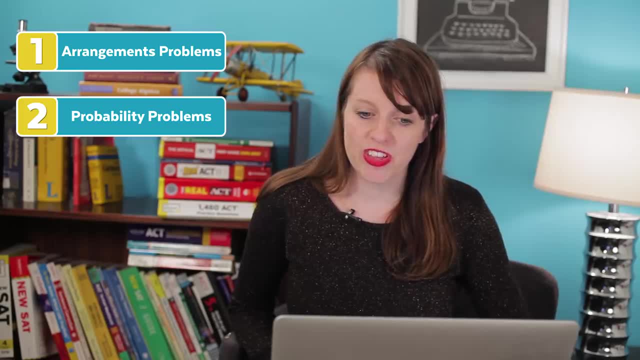 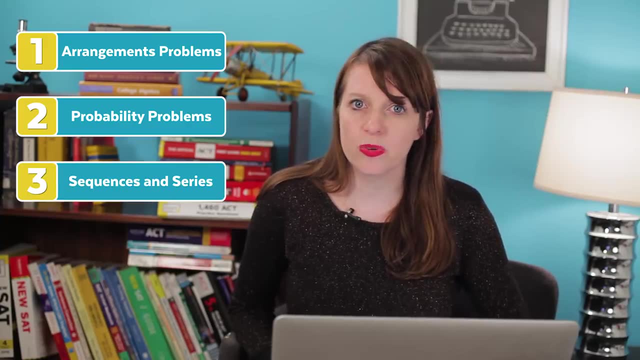 there's a whole in what those prep materials cover. So make sure that you have those probability problems down, Sequences and series, like I mentioned before. that's another area you need to work on Vectors. occasionally there are vector problems And matrix multiplication and 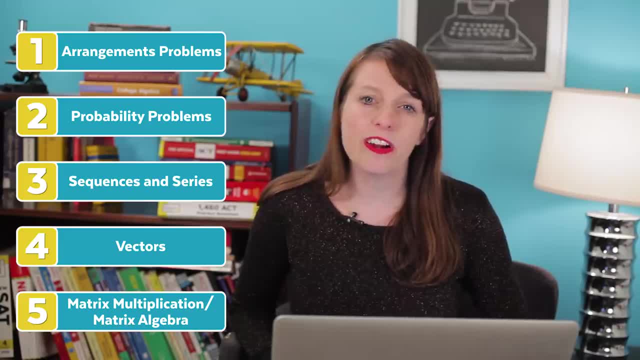 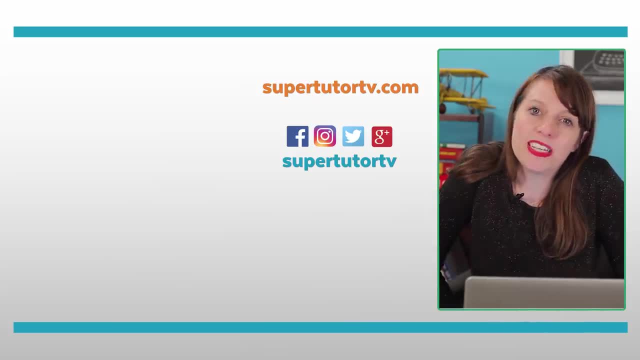 matrix algebra. So that's about it. Those are some other areas that you might want to work on if you want to work on the toughest kind of problems that are math on the ACT. I hope you guys like this video. If so, please give it a thumbs up. Subscribe to our channel by clicking.